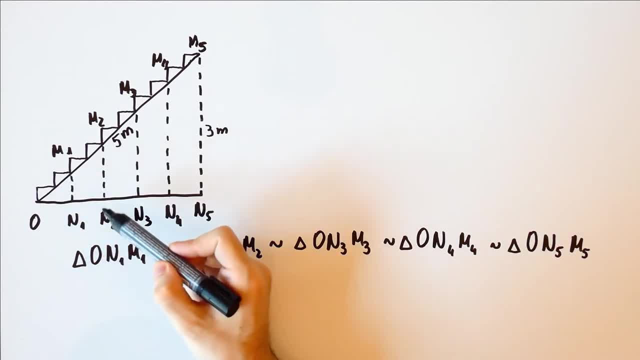 that N1, M1 over O M1 is equal to N2, M2.. O M2 over O M2 and that will be equal up to N5, M5 over O M5.. But O M2 over O M2. 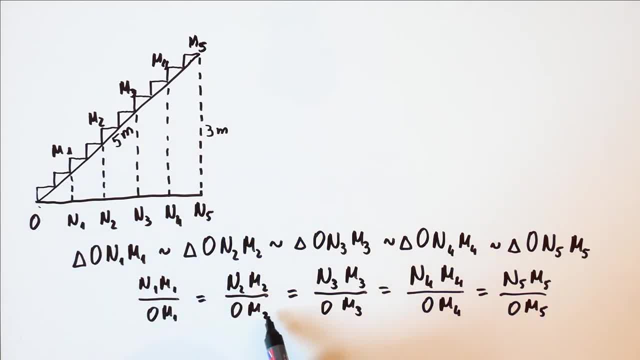 is 2 times O M1, so O M2 is 2 times O M1, which means that N2, M2 will also be 2 times N1, M1.. Similarly, O M3 is 3 times O M1, so N3, M3 will be 3 times N1, M1. 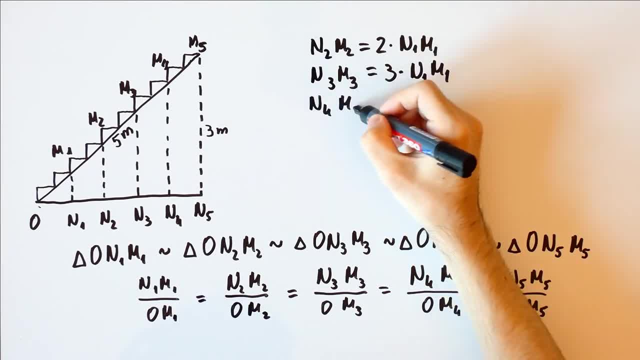 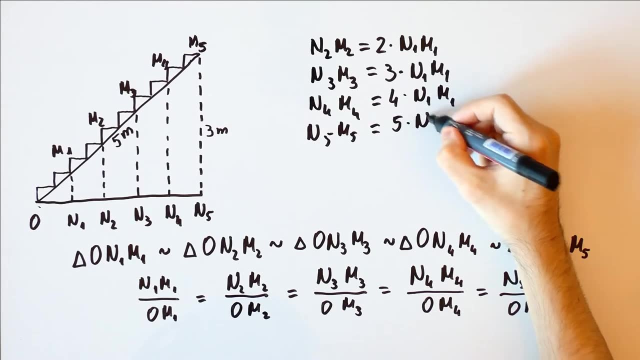 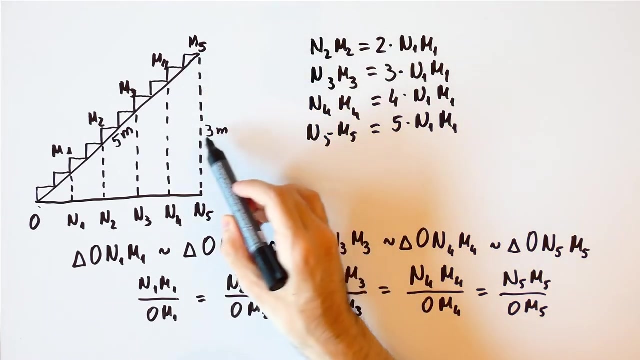 And N4, M4 is 4 times N1, M1. And N5, M5 is 5 times N1, M1.. But we know that N5, M5 is 3 meters, which means that N1, M1. 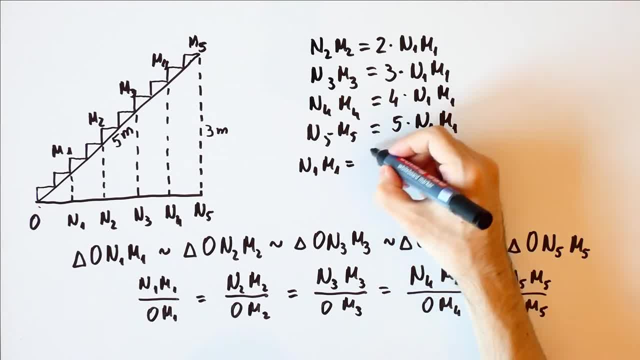 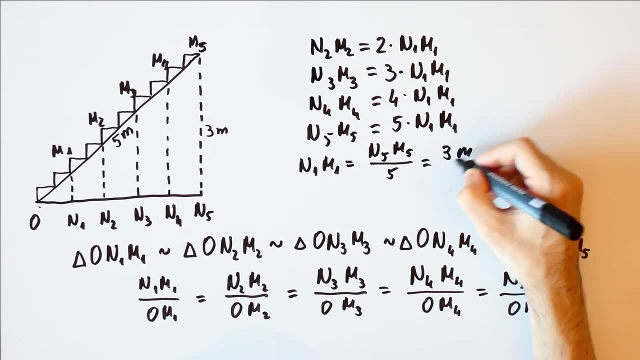 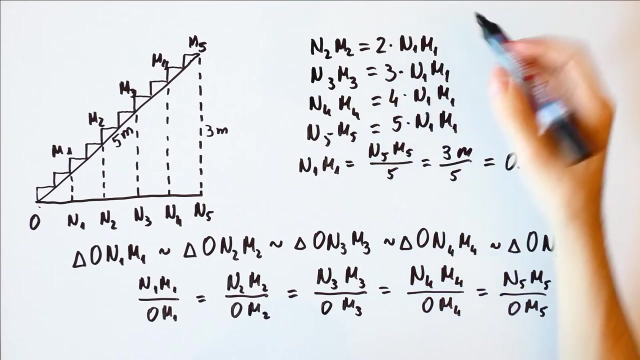 is equal to N5, M5 over 5, which is equal to 3 meters over 5, and that is equal to 0.6 meters. And now that we know N1, M1, we can calculate N2, M2, which is equal to 2 times N1, M1 and. 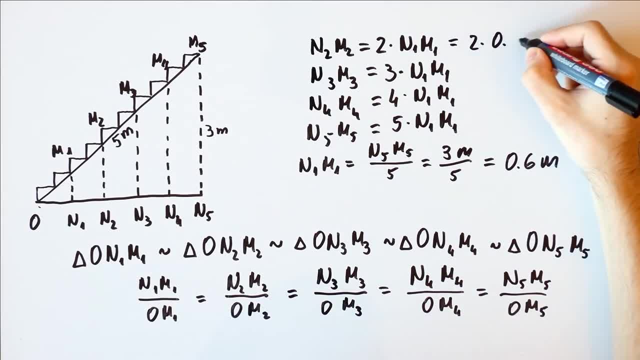 that is equal to 2 times 0.6 meters. which is 2 times 0.6 meters is equal to 1.2 meters. N3M3 is equal to 3 times 0.6 meters, and that is equal to 1.8. 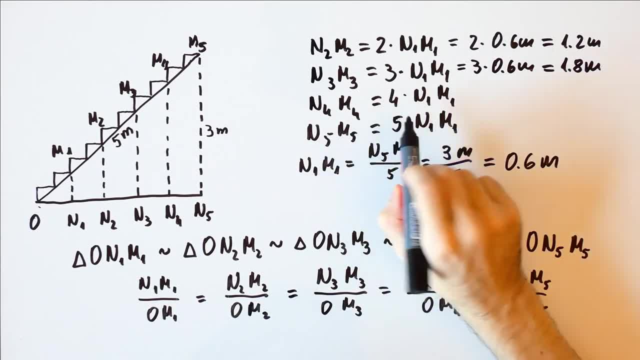 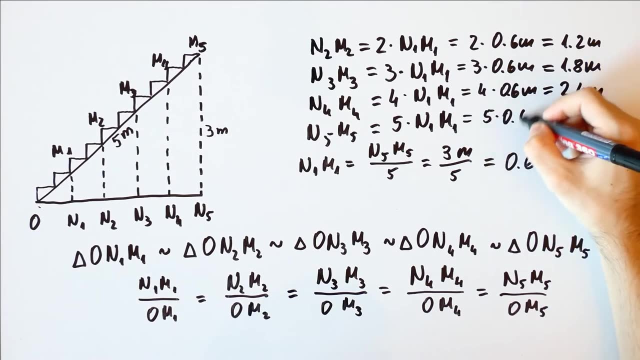 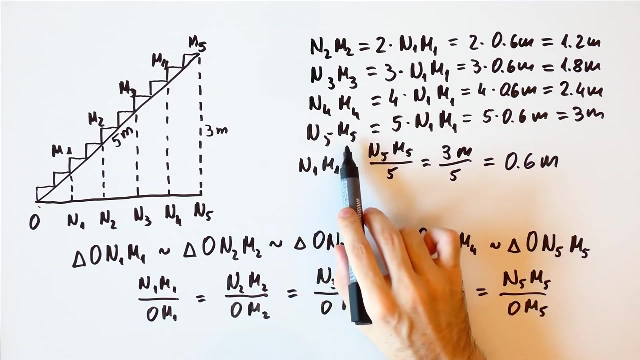 meters. N4M4 is 4 times 0.6 meters, which is equal to 2.4 meters, and N5M5 is 5 times 0.6 meters, which is equal to 3 meters. But of course we already knew that N5M5 is equal. 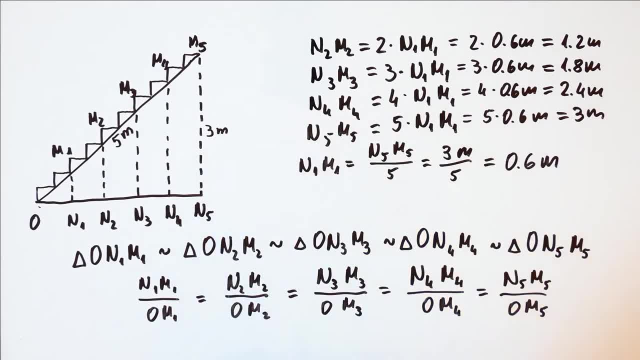 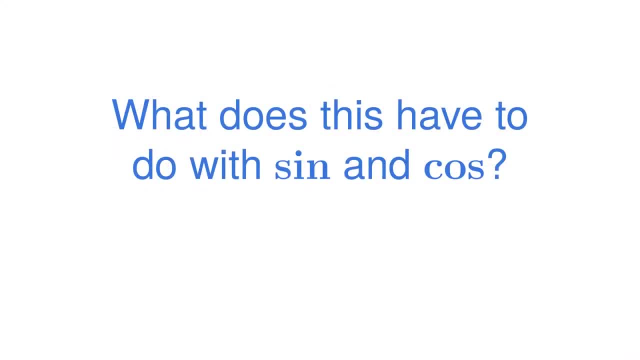 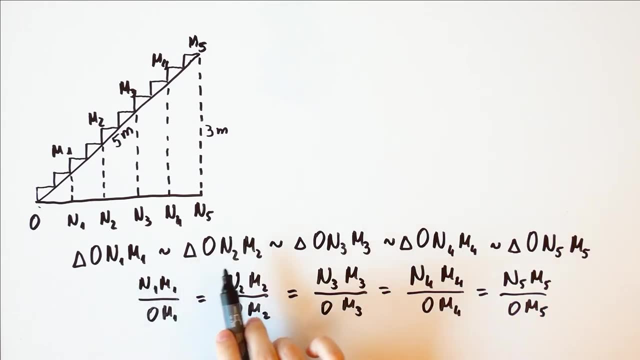 to 3 meters since that was given. What does this have to do with the sine and the cosine? We saw that these ratios are equal, and that is always the case when we have similar triangles. However, in this particular case, those triangles are right triangles and we say that the sine. 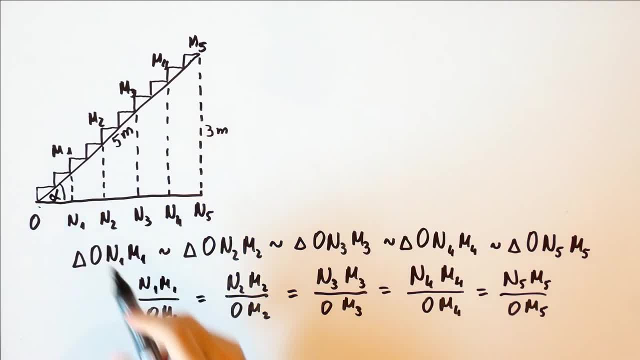 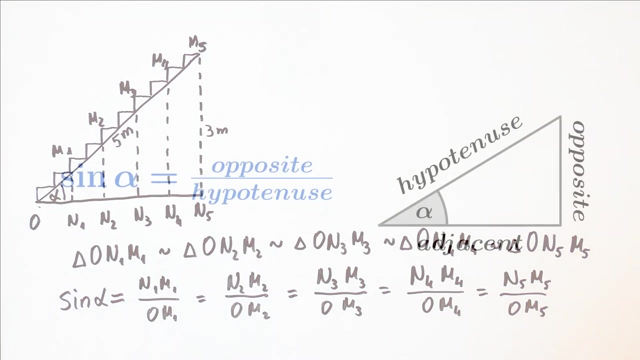 of this angle that we shall call alpha is equal to these ratios. And note that the sine of alpha doesn't depend on any particular triangle, since for all similar triangles the corresponding ratios are equal. Now we can define that if in a right triangle alpha is an acute angle, the sine of alpha 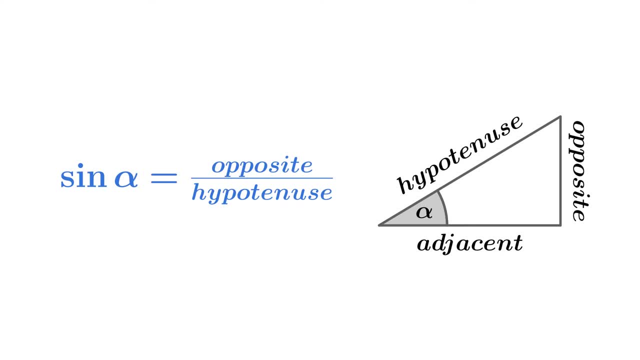 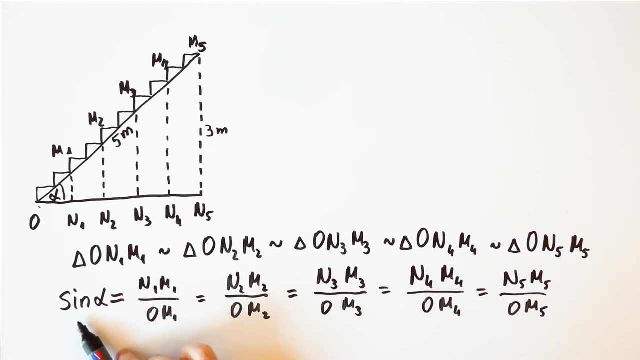 is equal to the ratio of the opposite leg to the hypotenuse. So what is the sine of alpha in our example? Well, the sine of alpha is equal to these ratios and in particular, it's equal to N5M5 over OM5.. 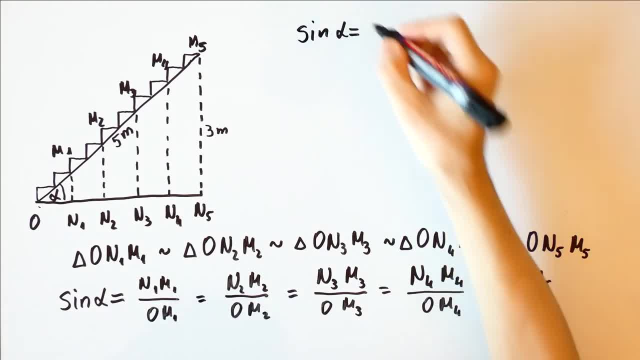 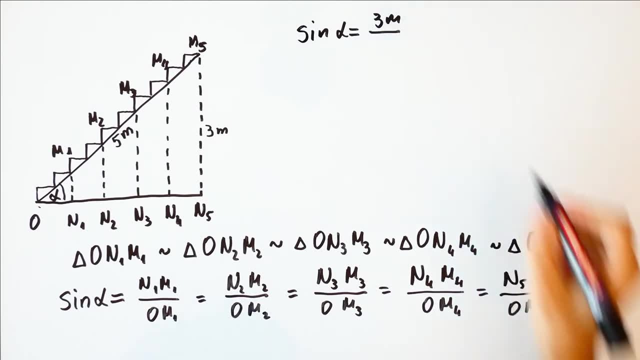 So the sine of alpha? The sine of alpha is equal to N5M5,, which is 3 meters, over OM5, which is 5 meters, and that is equal to 0.6.. And note that the sine of alpha doesn't have any unit. there are no meters or degrees. 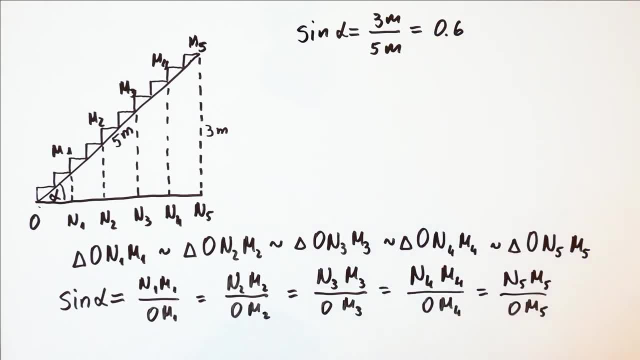 or any other unit. it's just a number. But can we somehow use the sine of alpha to calculate the heights of these supports? Well, for support N1M1, we can say that N1M1 is equal to the sine of alpha times OM1.. 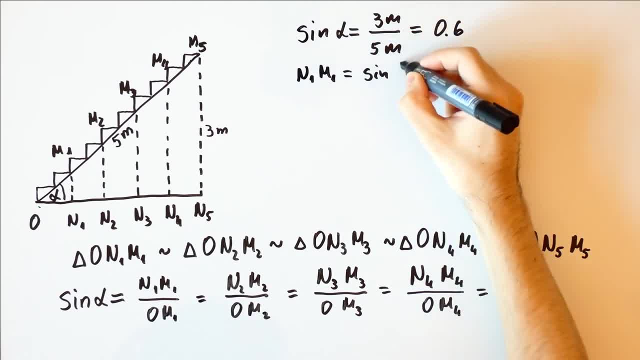 Similarly, N2M2 is equal to the sine of alpha times OM2.. Ok, So let's do this: N2M1. N2M2. times OM2.. And N3M3 is equal to the sine of alpha times. 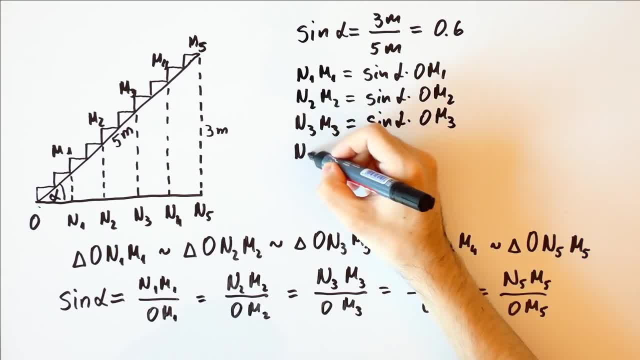 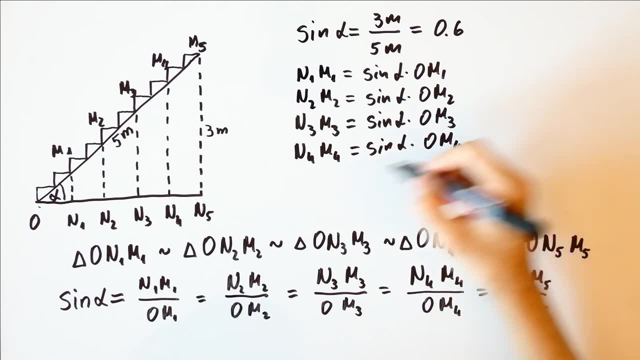 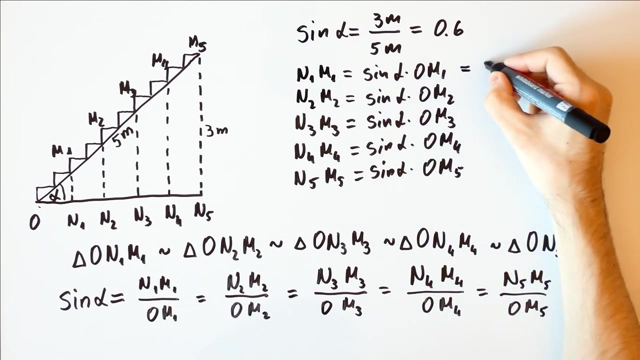 OM3.. N4M4 is equal to the sine of alpha times OM4.. And N5M5 is equal to the sine of alpha times OM5. But the sine of alpha is equal to 0.6 and OM1 is equal to 1 meter. 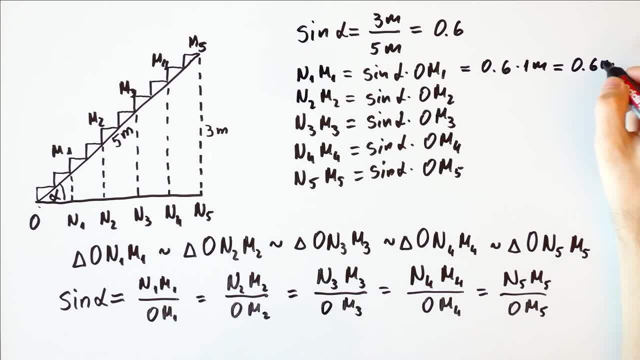 So this is equal to 0.6 meters. For N2M2, we get that this is equal to 0.6 times OM2, which is 2 meters, and that is equal to 1.2 meters. N3M3 is equal to 0.6 times 3 meters. 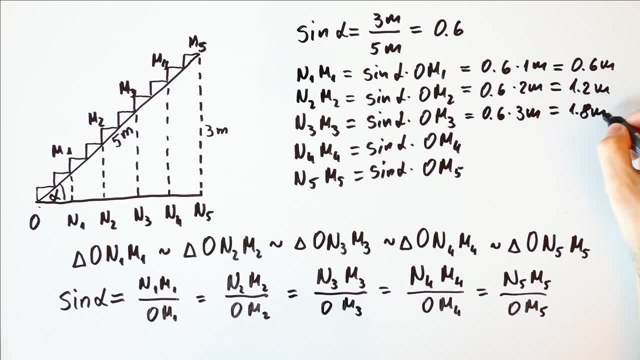 and that is equal to 1.8 meters. N4M4 is equal to 0.6 times 4 meters, and that is equal to 2.4 meters. Therefore, N2M1 and N4M4 are excraelingly equal. 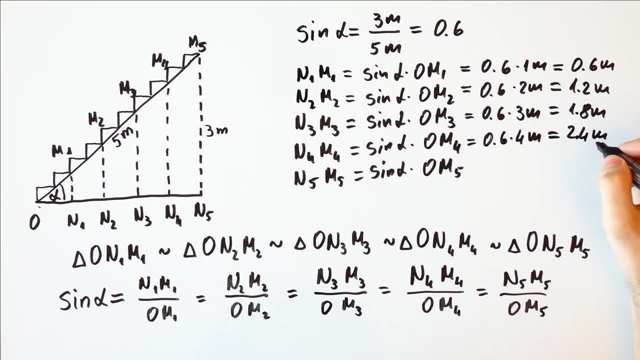 We will see the difference in values And starting from T pressed symbol. thank you, H gr. Thank you A meters and n5m5 is equal to 0.6, times 5 meters and that is equal to 3 meters. 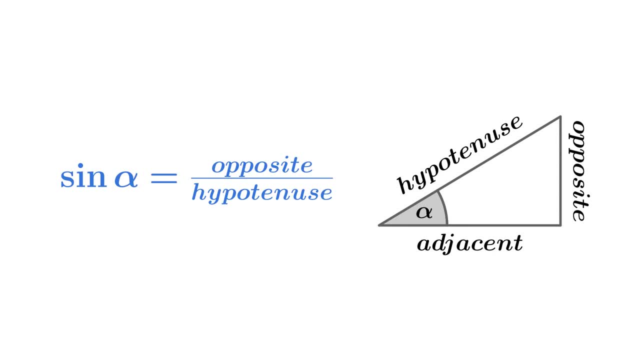 If the sine of an angle is equal to the ratio of the opposite leg to the hypotenuse, what is the cosine? Well, the cosine of an angle is equal to the ratio of the adjacent leg to the hypotenuse. We started with a problem concerning heights of supports of stairs and whether we have 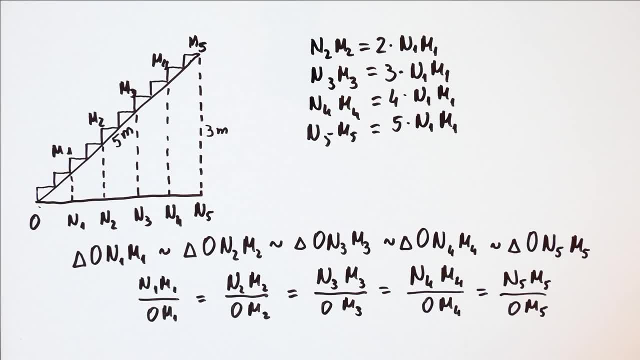 to measure each of them. Then we noticed that we have similar triangles and that the corresponding ratios are equal, And from those ratios we were able to calculate the heights of supports. Now, in that particular case, the ratios we observed were between legs and hypotenuses. 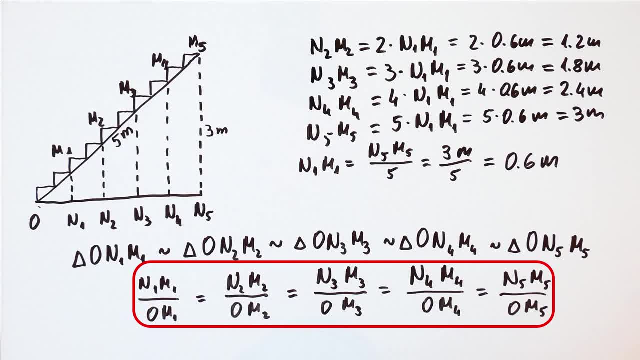 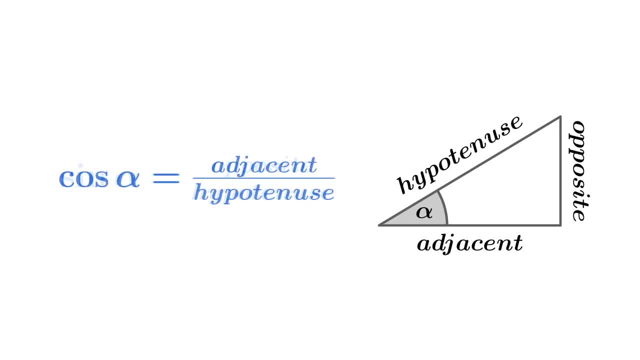 of right triangles, which is how we define the sine of an angle, Namely as the ratio of the opposite leg to the hypotenuse. Similarly, the cosine of an angle is defined as the ratio of the adjacent leg to the hypotenuse.